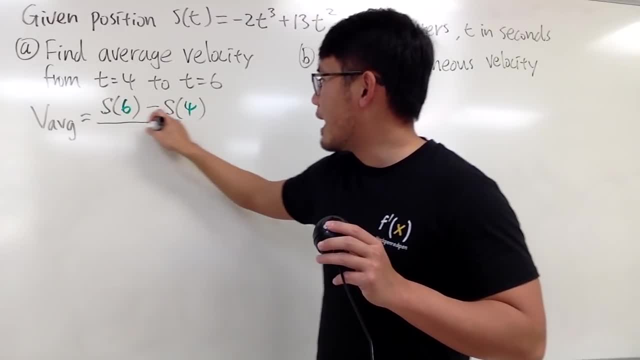 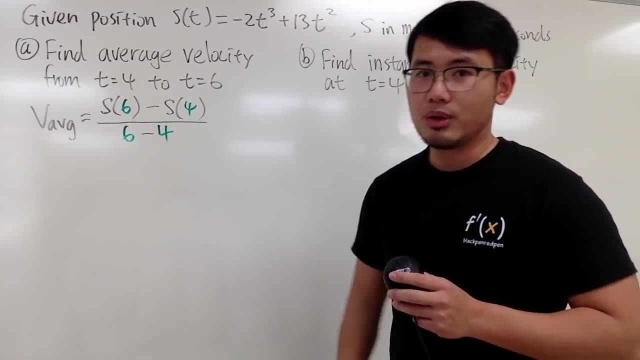 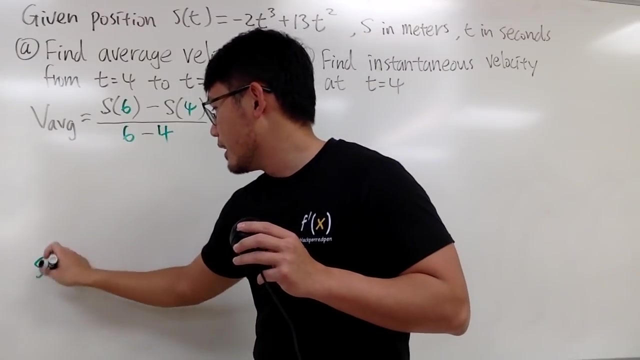 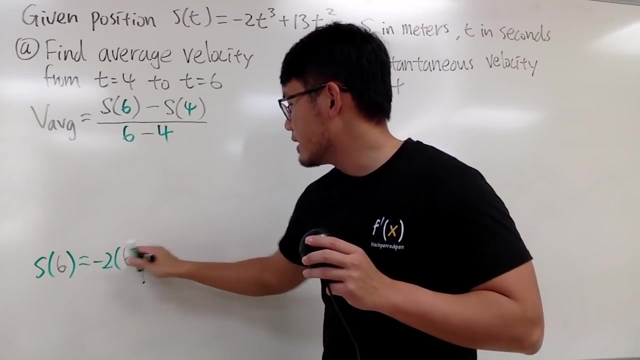 Because that will be the initial position, And then divided by how long it takes, right, So it will be 6 minus 4, which is 2 seconds. But this is pretty much all you have to do, Well, to get s of 6, you refer back to this equation And let's just put it down right here real quick: s of 6, this is equal to you: put 6 into the t's, you get negative 2 times 6 to the third power and we add 13 t squared, So that's plus. 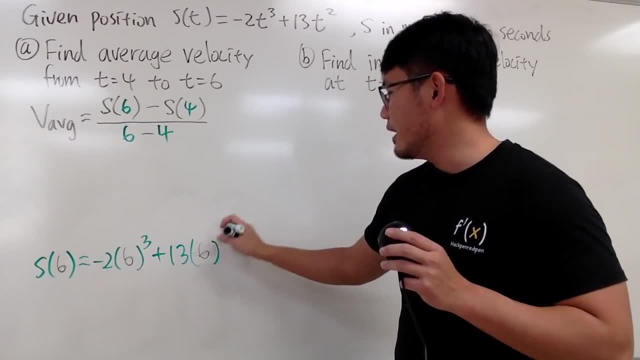 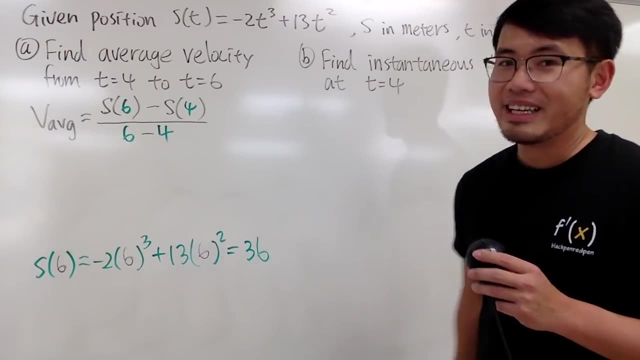 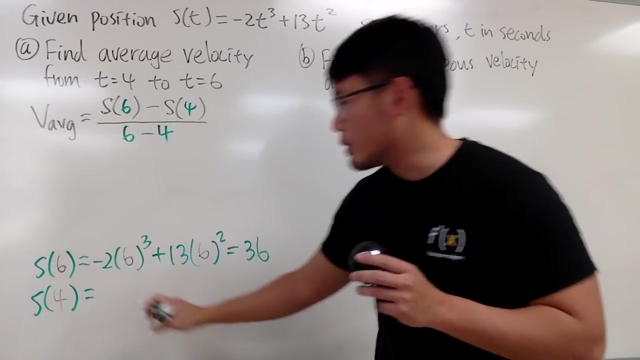 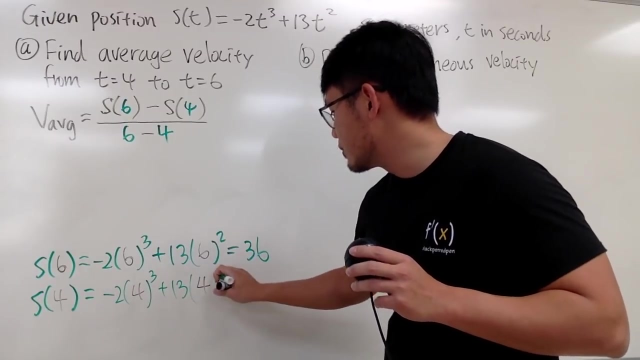 13 t squared And the t is 6.. So put the 6 here, and then we have that square. Of course, right here you can just work this out, I will leave that to you. you end up with 36.. And then, similarly, we calculate s of 4 by putting the 4 into all the t's right here. So we end up with negative 2 times 4 to the third power, plus 13 times 4 to the second power, and you end up with 80.. Well, well, right here we can come back. 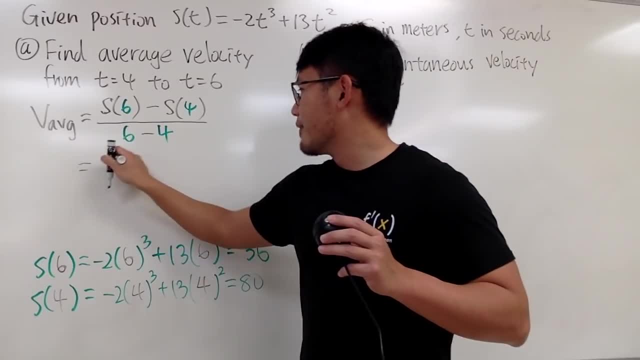 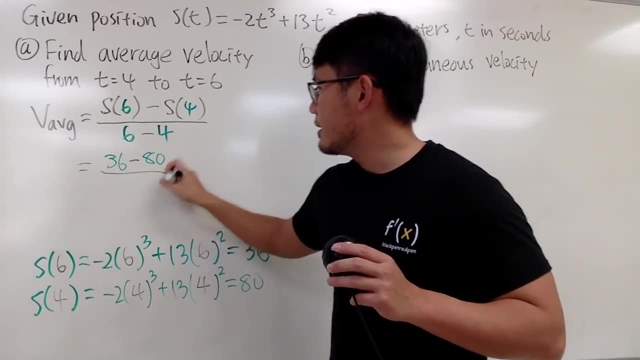 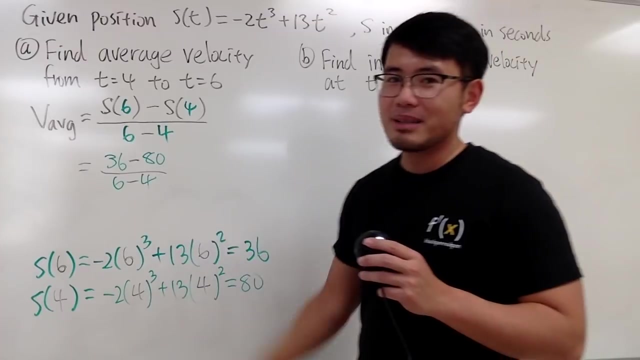 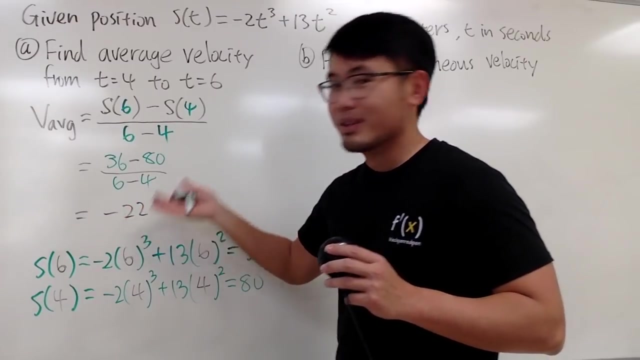 s of 6 is 36.. And then we minus s of 4, which is 80. And over. let's just keep it at 6 minus 4, which is of course 2.. But just do this on your own. On the top it's negative 44, on the bottom it's 2.. So altogether you end up with negative 22,. right, This negative 44 divided by 2.. So negative 22.. And notice the s, which is the position is: 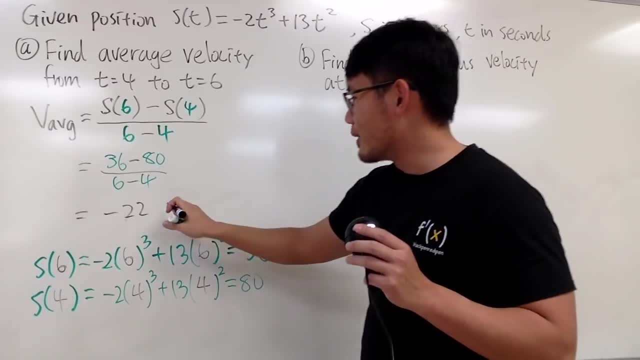 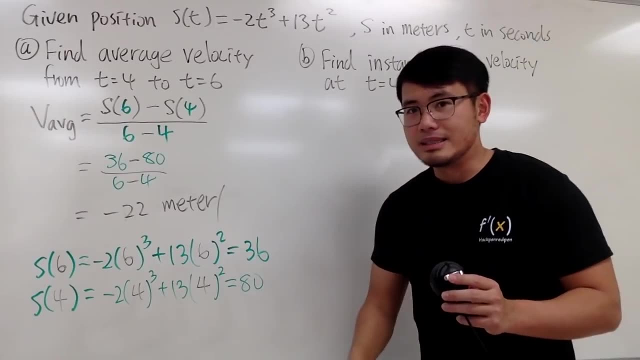 in meters and then t is in seconds. So right here I already done as meters per second. But let me spell the out, because sometimes if you abbreviate the s as second or the position is, I don't know. 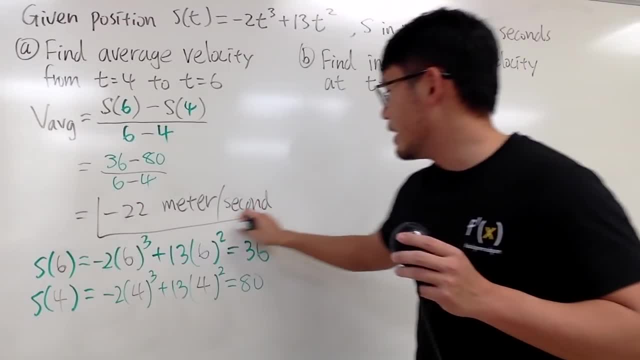 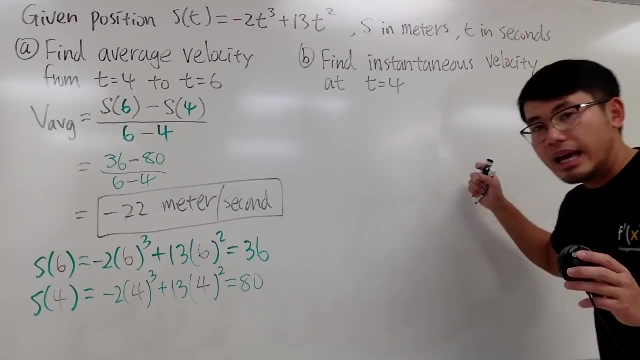 seconds. right, Yeah, so that's it. And here you have negative velocity. that means you are, you know, on average moving toward the left, All right. On the other hand, if you want to find the instantaneous velocity of the moving particle when t is 4,. 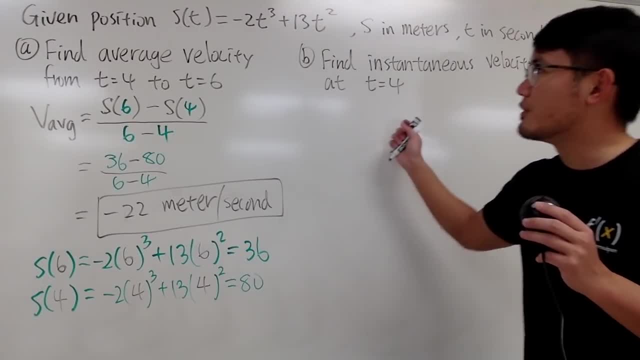 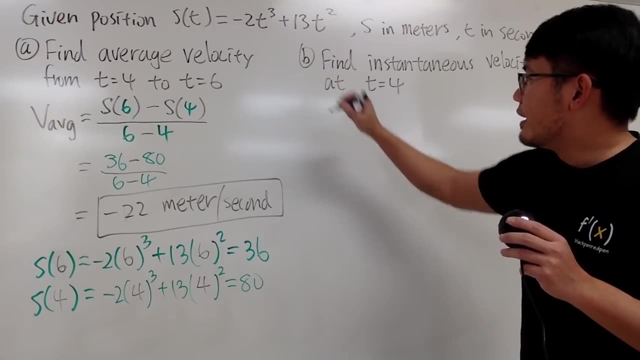 we have to do this. So we end up with negative 4 times 4 to the third power plus 13 times 4 to the second power. Do some calculus, then you can just do the derivative, because the first derivative tells you the instantaneous velocity. All right, So right there, I will just try down. phi of t.